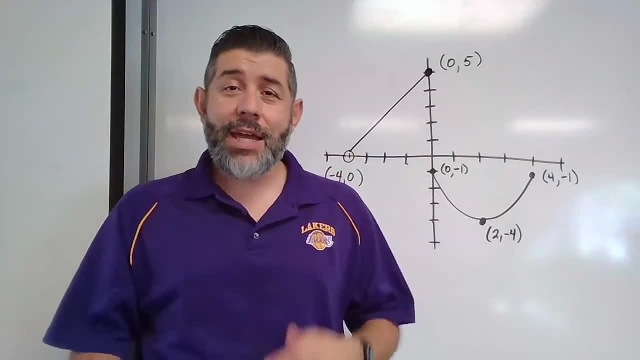 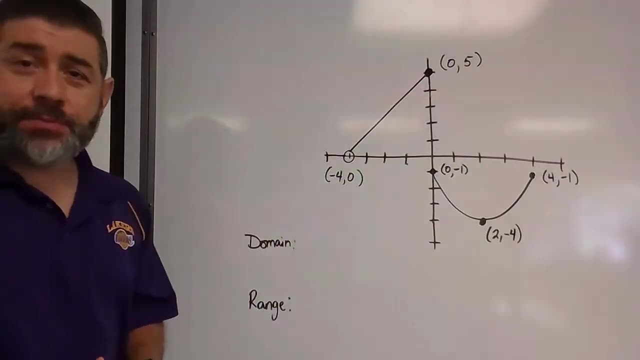 to figure out domain and range, a piecewise function and a rational function. But we're just going to look at the graphs, all right, And we're going to write these at interval notation. So take a look at this graph here. You want to pause it? Go ahead, Pause it, Freeze And then 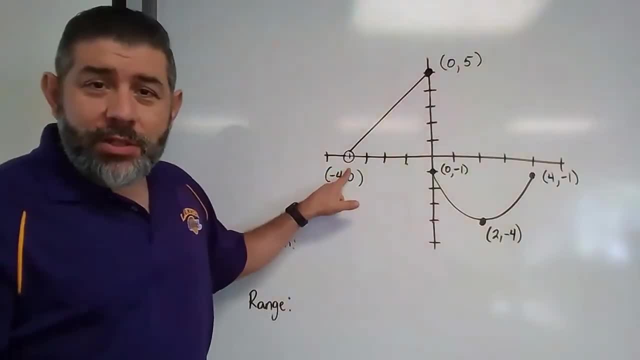 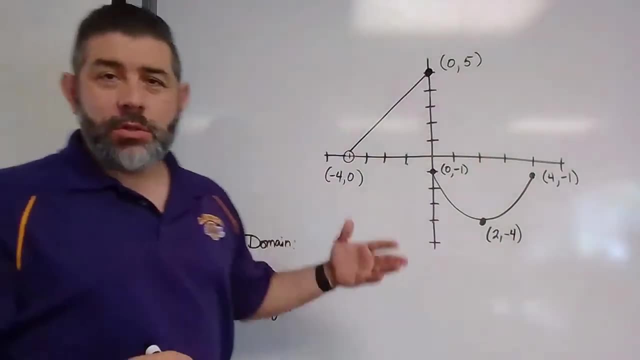 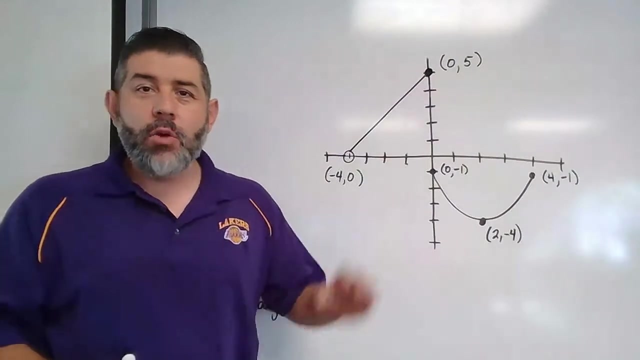 move on, Here we go. So I want you to notice right here: this is an open circle, all right. Open circle means that it is not included, not included in our graph. Closed circles mean that they are included. So the domain. the domain is about the X values. all right, We're looking. 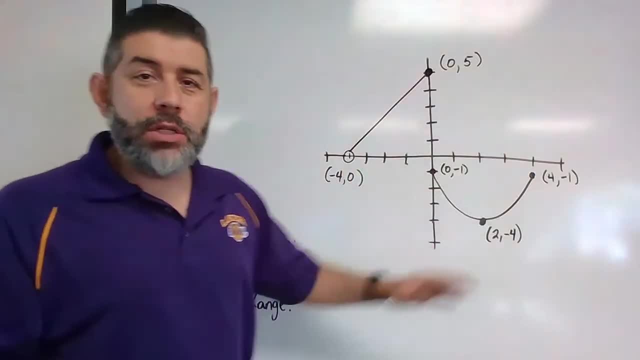 on the horizontal axis left and right. What we're going to do is we're just going to look at the X values. all right, We're going to look at the X values, all right, We're going to start here and we're going to keep like we're going to slide over until we 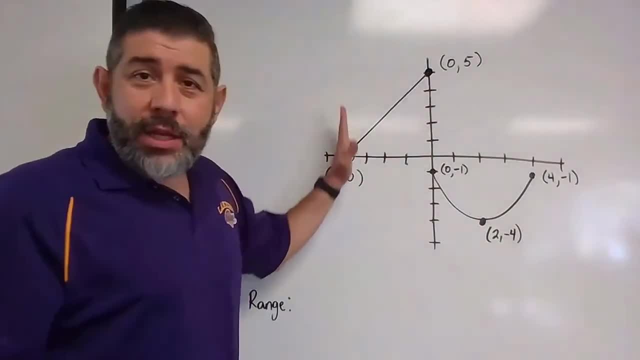 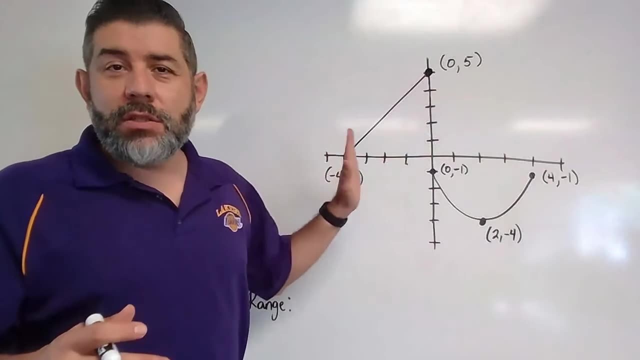 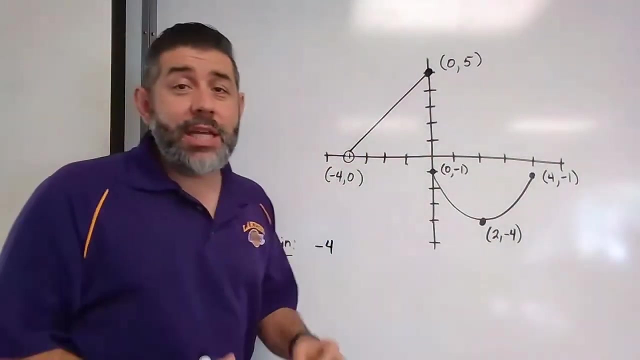 get to our first piece of the graph up right there: Negative four on my X. that's where it starts, Even though it's open. that's where my graph starts to hit my hand once I go around there. So I'm going to start this at negative four. We're always going to go left to right. Now we're using 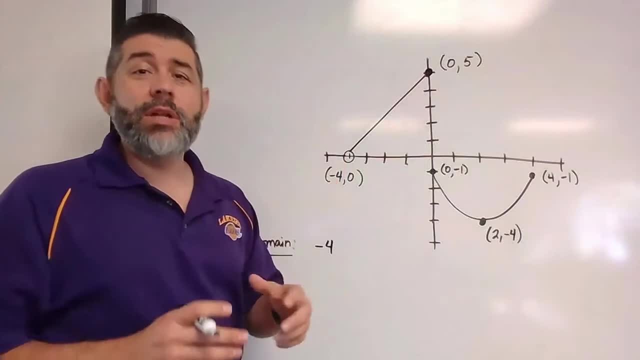 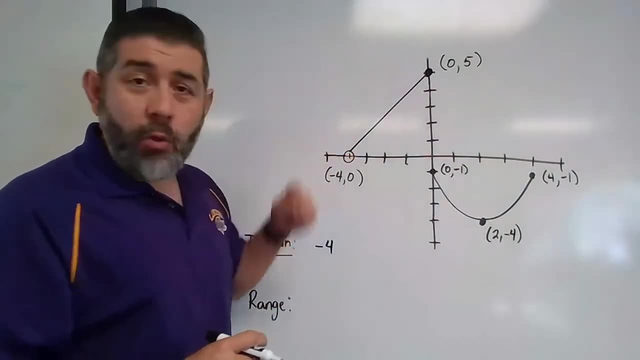 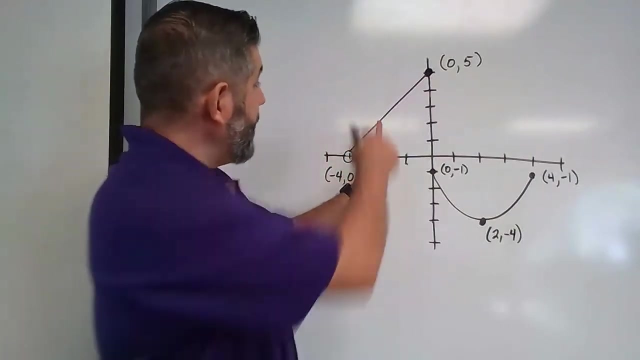 interval notation. So we use a parentheses when a value is not included and a bracket when the value is included in our graph. Since this is an open circle, I'm going to make a parentheses. Now I'm going to continue The graph. the graph is still hitting my feet, my hands here, right, 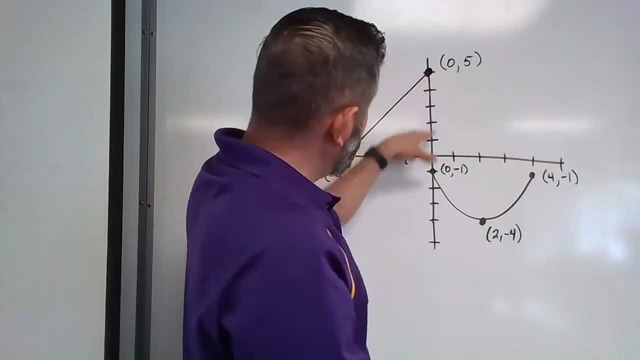 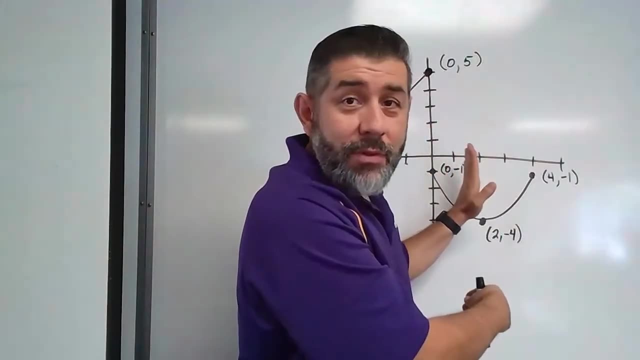 The graph's still hitting my hands. I still have X values. There's still X, even though there's a break here. the X value zero. it's still hitting my hand right. It's still hitting my hand. Still, it's giving me a high five. Xs are still giving me high fives all the way until you get to here. 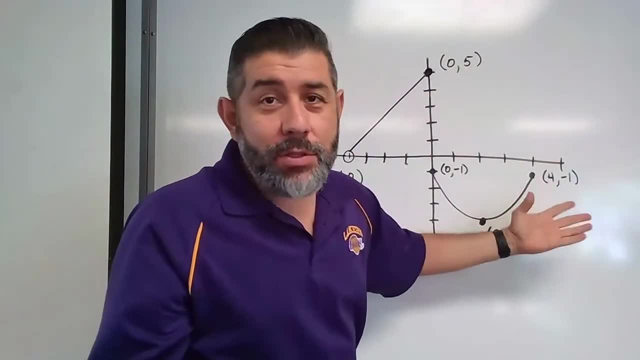 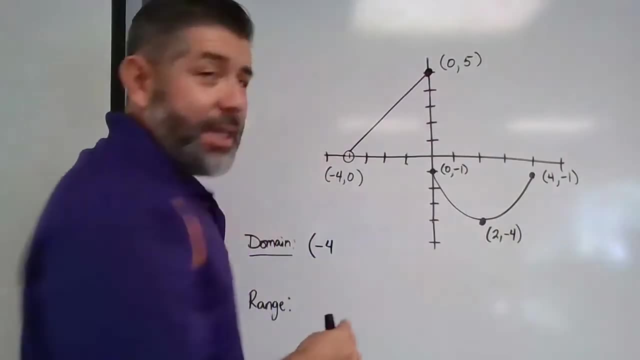 Once I pass positive four, there's no more right. It rhymes, There's no more graph. So four is kind of our ending, but it is our ending place. In fact it's a closed circle. So we're going to go four. 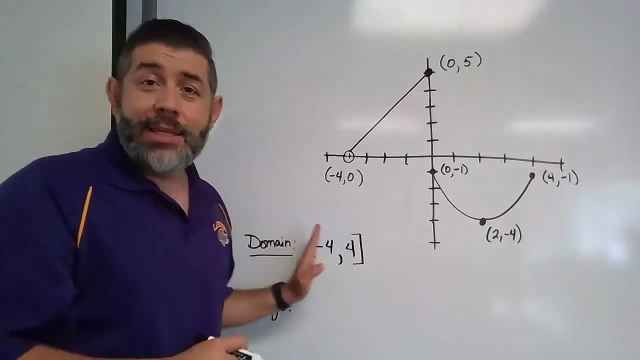 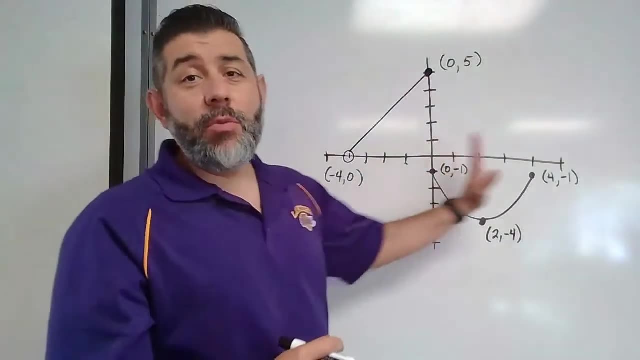 negative four to positive four and a bracket, and this would be our domain. all right, Now our range goes up and down. So, just like I went left and right for my Xs and my domain, my range is going to go from the bottom up. 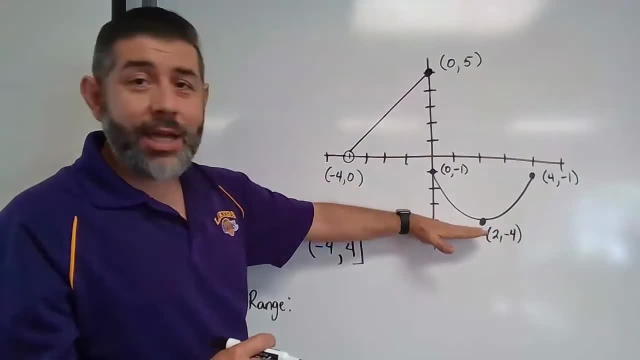 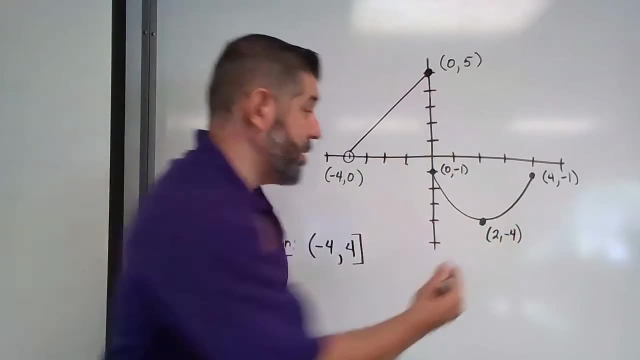 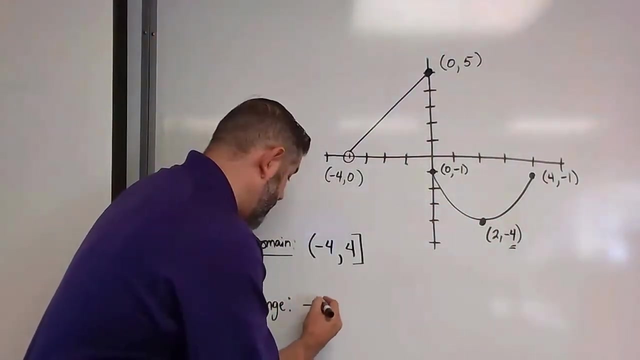 to start down here. I'm going to do the same thing with my hand. I'm going to slide up until I get to the first point. first point is a y value. I'm looking at the y values now of negative four. that's the first part that touches my hand of this graph. so I'm going to say negative four. 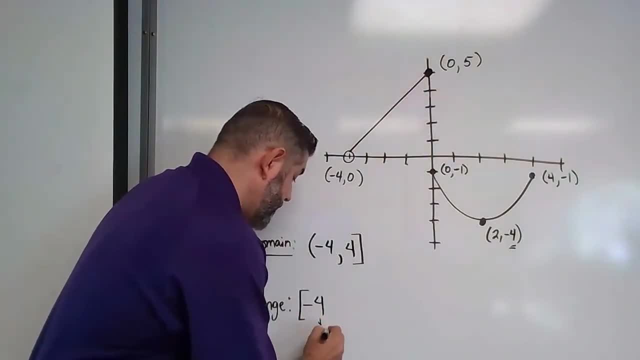 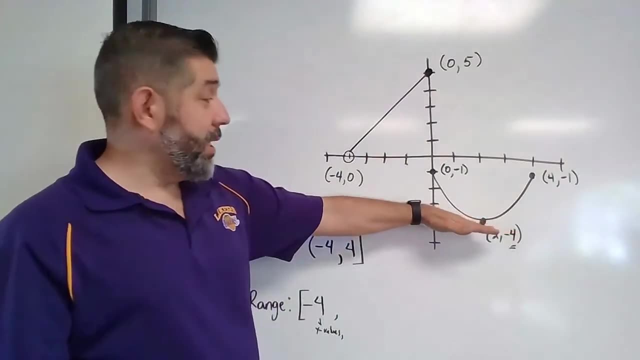 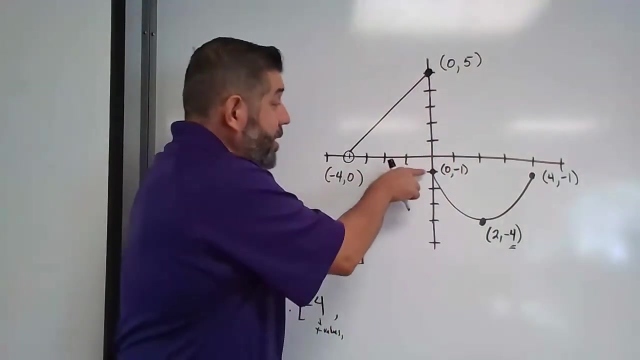 all right, this is again. these are the y values. y values, all right, so I'm going to go to negative four here. that's my y value. I'm going to keep going. it's all touching my hand. it's still touching my hand, still touching my hand, still touching my hand here. but look right in between. 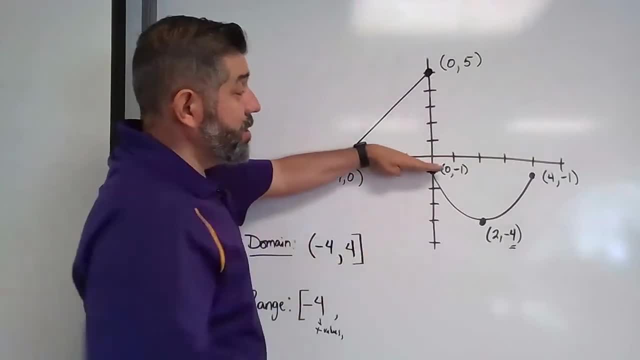 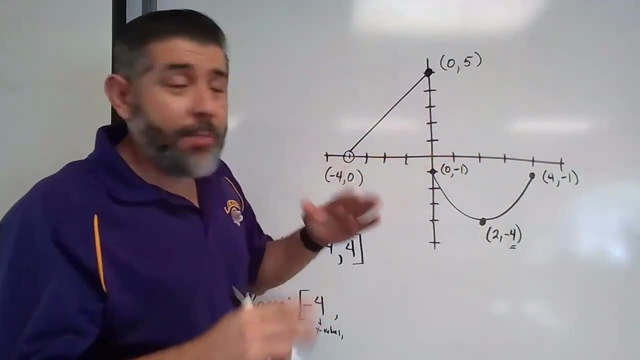 here and here there's a little break, like there's nothing touching my hand here, so I have to. I have to account for that. so as soon as it stops touching my hand, I'm going to have to stop it there. so it's it's going to be at negative one is my y value, so I'm going to go to negative one. 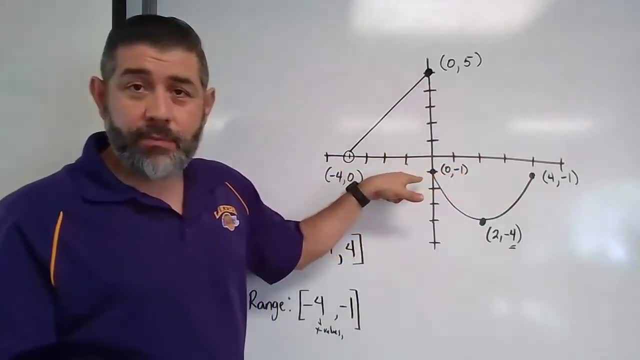 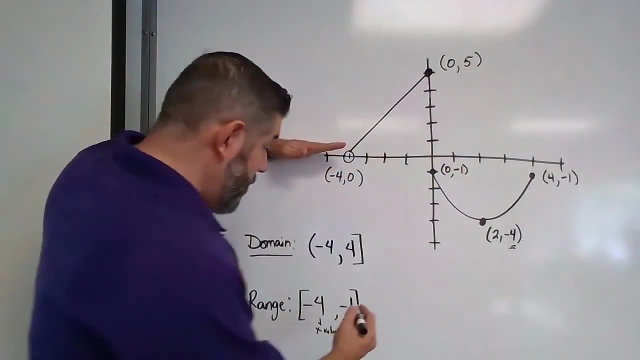 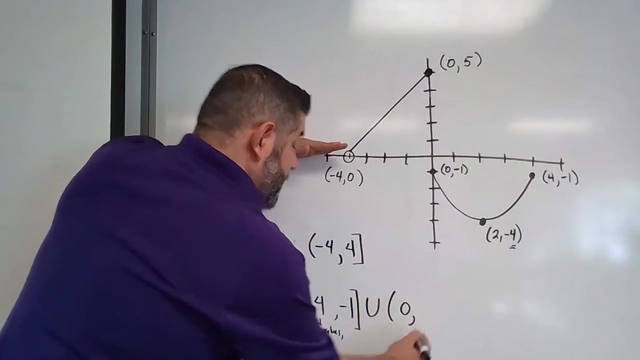 and I'll put bracket because these are solid. now I'm going to keep going, and now there's nothing, nothing, nothing. then it touches my hand again at y equals zero. so i'm putting a big u here. u means union, and i'm going to open parentheses zero, because that's where i'm. 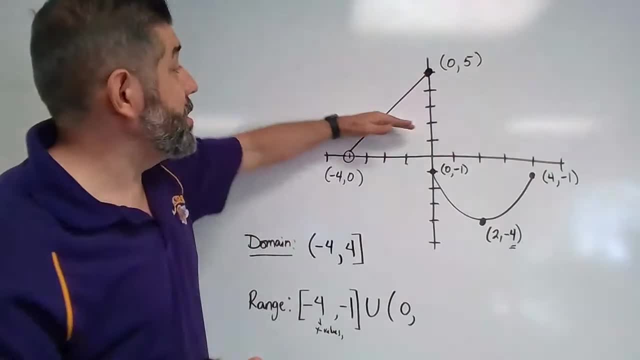 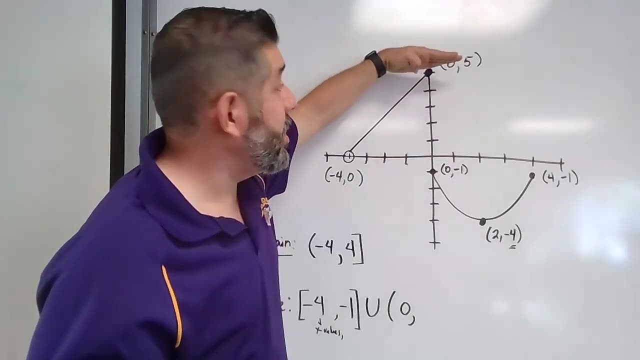 starting again, starting at the y zero. then i'm going to go up and up and up. it's still see, it's touching, it's touching my y, my hand still touching the graph, and then up right there after that, no more touch, no more touch. so this is going to go up to five and that's going to be a bracket, because 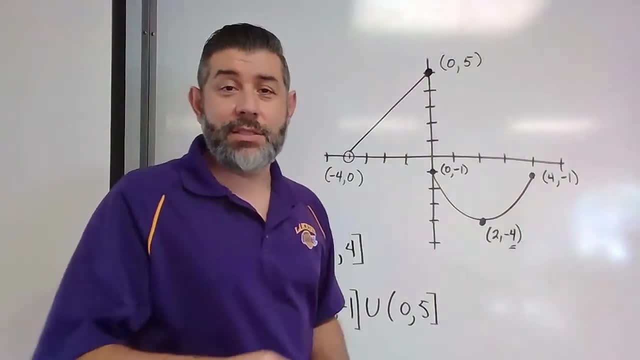 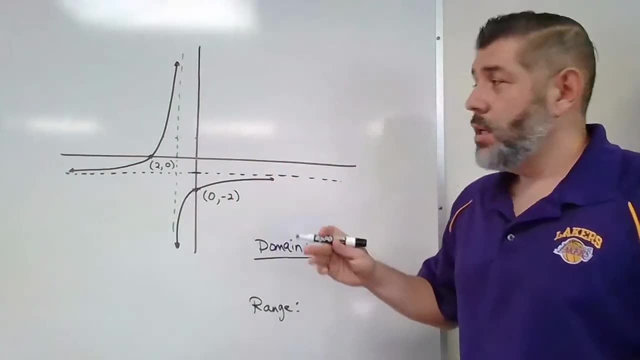 it's closed. all right, so let's take a look at the next example. all right, here's our second example, which is a. it's a rational, okay. it has two what we call asymptotes, so we've got a vertical asymptote here and a horizontal asymptote here, and what that means is the values are going to go out to. 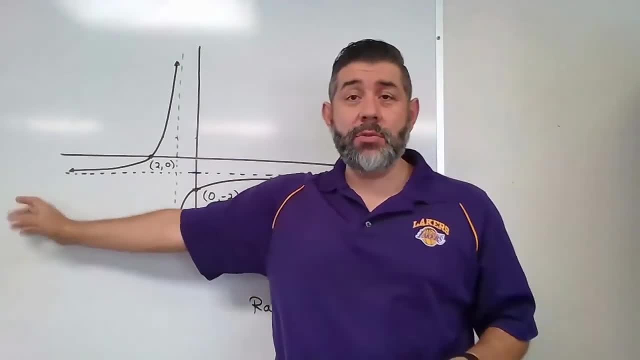 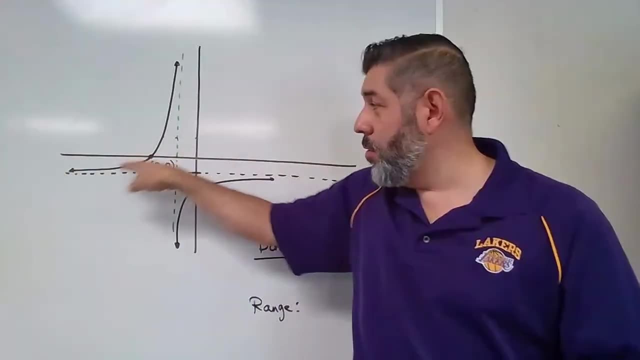 infinity. so this is what this looks like. we're going to again. we're going to for domains we're going to look at horizontally, so from the left to the right, all right. so we're going to start here and notice this arrow goes all the way up. that means it goes forever. so forever in the x direction, in that way, on on. 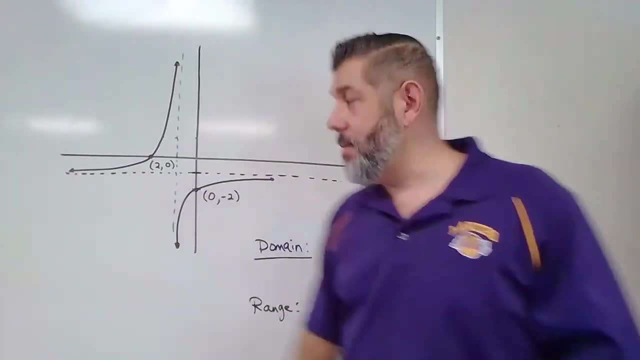 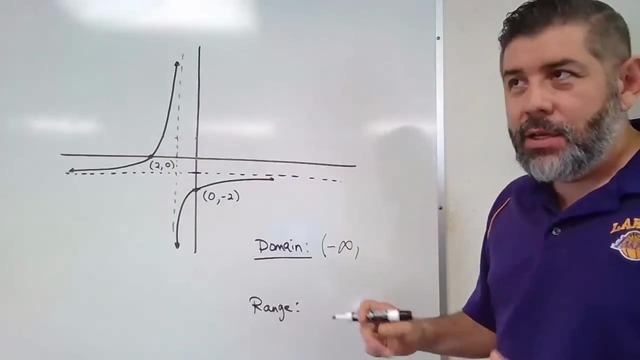 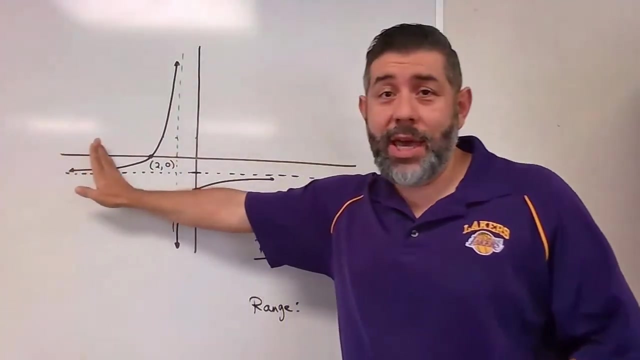 horizontally forever. that's negative infinity. so my domain is going to be negative infinity. now we don't include negative infinity. we put a parentheses because it's more of an idea rather than an actual number. so i'm going to go negative infinity and it's going to keep going. okay, x is x. 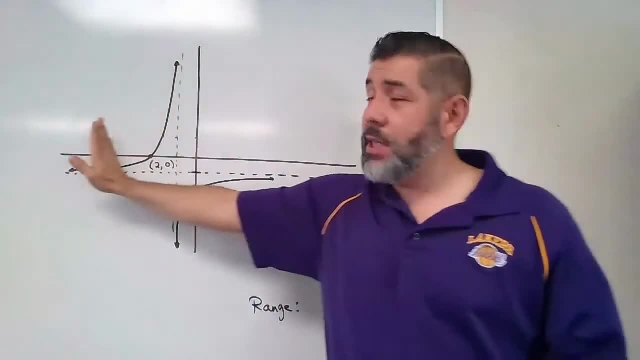 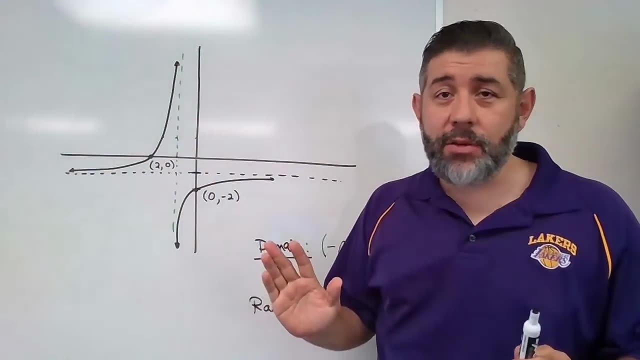 is. It starts to go up this way, but I'm not going to follow it up, I'm just going to keep my hand going this way. all right, It touches there, but then look right here at this asymptote: there's no x value there. 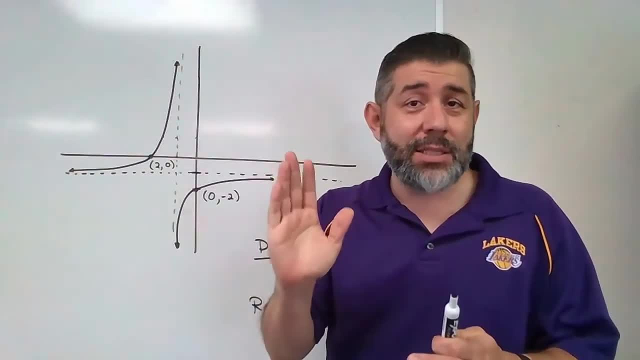 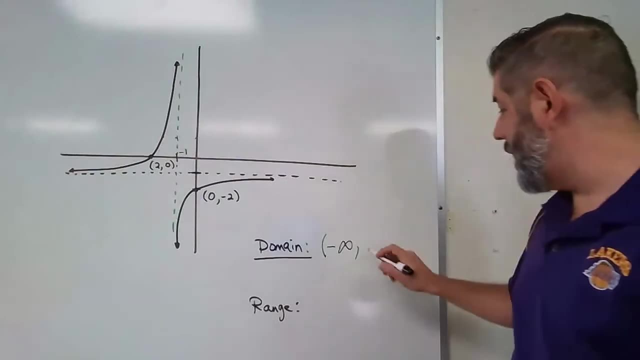 So there's no x value there. I have to stop there because it's not touching my hand technically, Remember, we're just going left and right, So this is going to be at. I forgot to mention that that's negative 1,. all right. 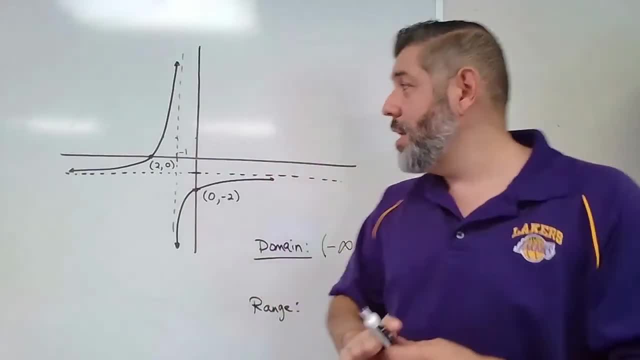 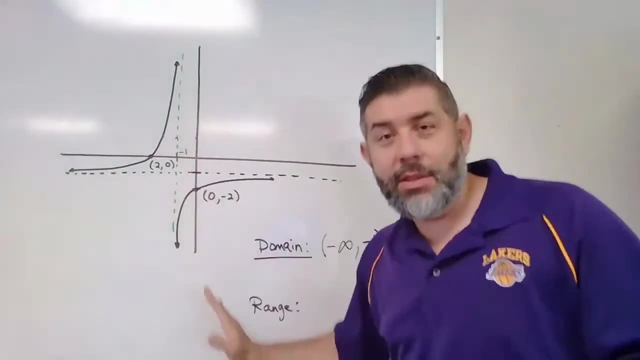 Then I'm going to close, I'm going to keep a parenthesis there because it doesn't touch. Then it's going to start again after it doesn't touch negative 1.. It's going to keep going. Remember, we're not going to go like this. 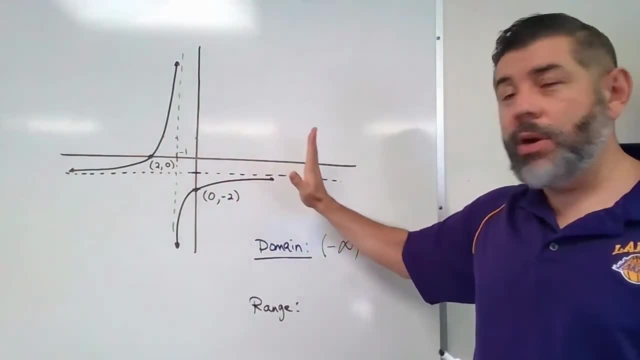 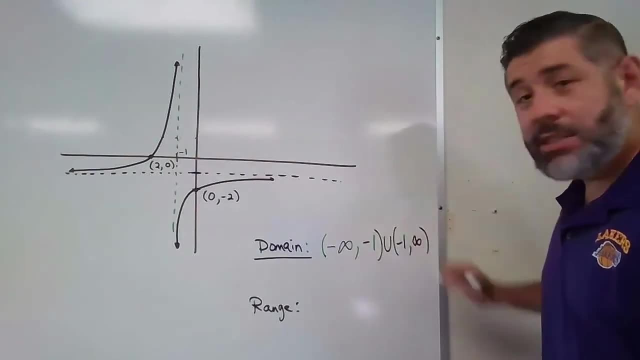 We're just going to follow our hand along this way, and now we're going to go all the way over to positive infinity. So we're going to union this again and we're going to go negative 1 to positive infinity. Our range is going to do the same. 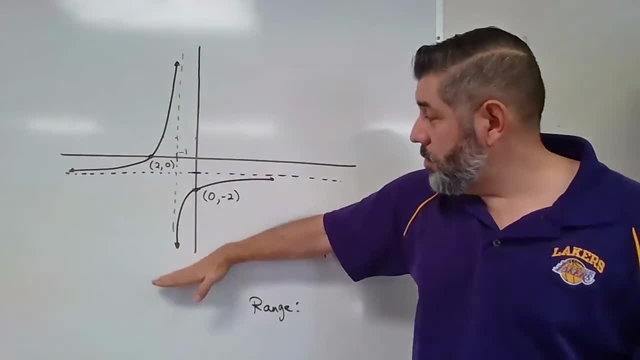 We're going to do the same thing. We're going to go down from the bottom up, okay? So I'm going to do this negative infinity again, because it's going down. It's going down forever, right? So I'm going to go negative infinity. 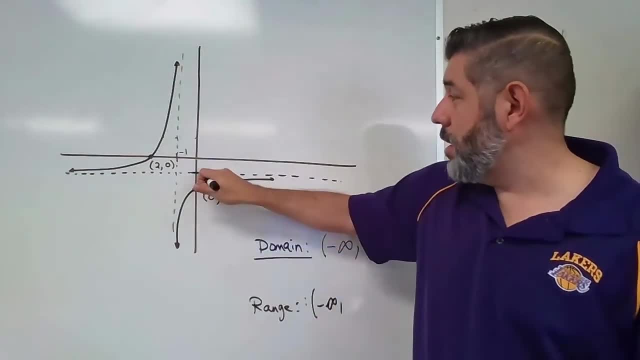 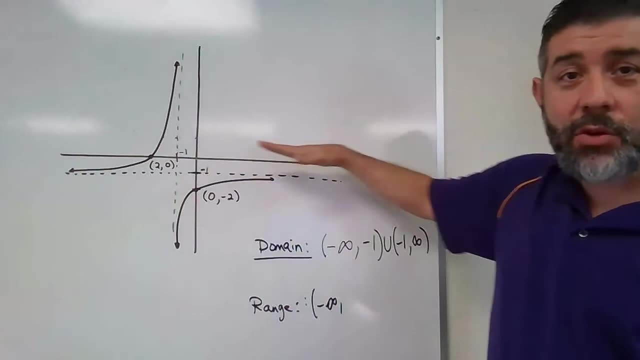 Now what happens? it's going to go up, go up, go up, and this is negative. 1 is my horizontal asymptote Notice here. I'm not going to follow it along like I did right Once I start to go this way. now I'm going x direction. 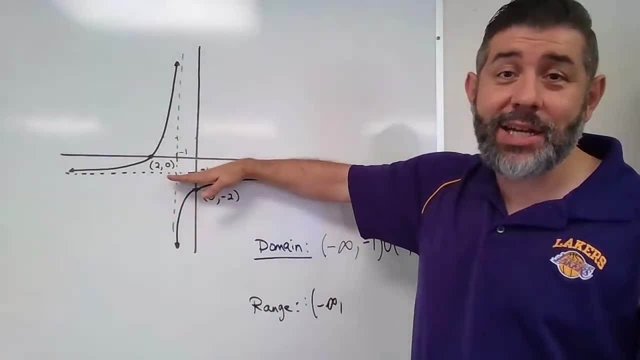 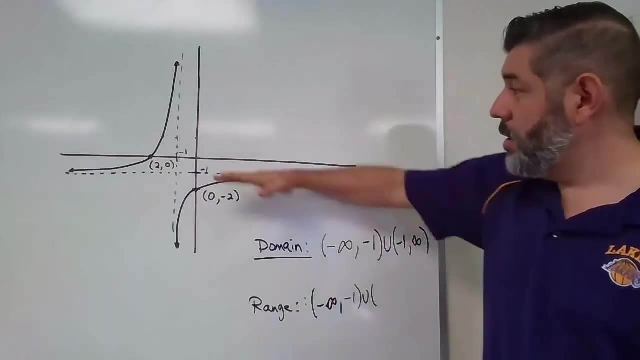 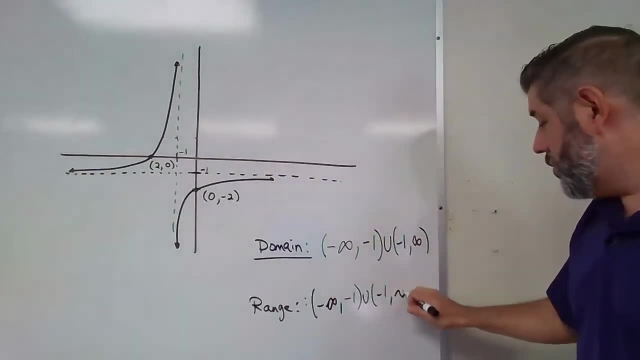 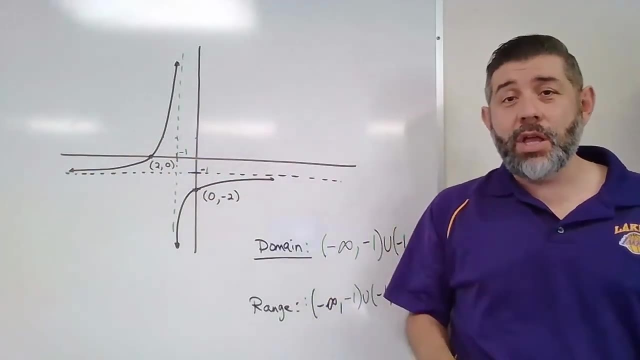 up and up and up. it goes up forever to infinity and beyond. All right, so you've got two examples there, one with a piecewise, another with a rational. Hopefully that makes sense, for how do you do domain and range graphically? 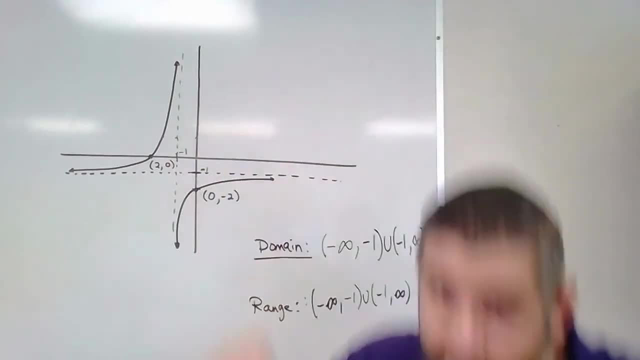 We'll see you next time, folks Maestas out.